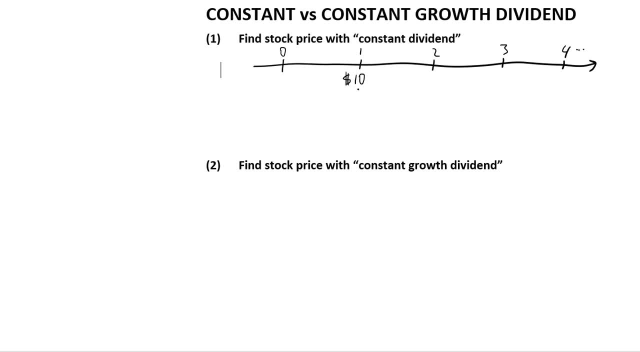 So you buy a stock share now. your first dividend will be in a year in the amount of ten dollars on your one share. Let's say we also know that the interest rate or the discount rate is twelve percent. This is what we are given Here in the 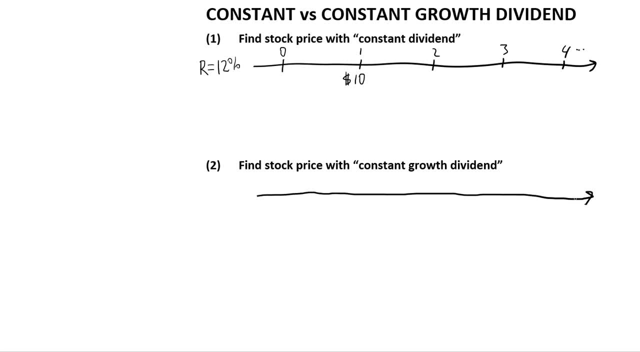 second case, we have exactly 12 percent. This is what we are given Here. in the second case, we have exactly 12 percent. This is what we are given Here. in the second case, we have exactly the same thing, except we will have one additional piece of information. So let's. 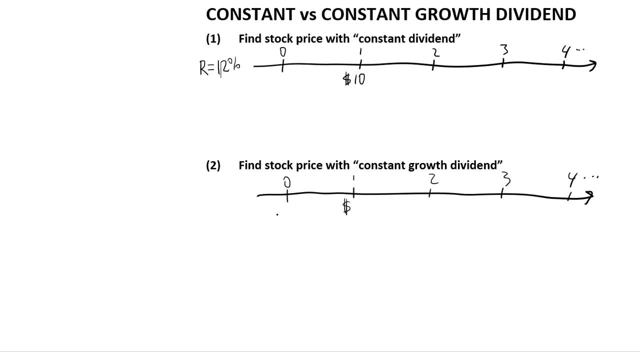 mark our years Again. if you buy a share of stock today, year zero, your first dividend will be ten dollars, paid in a year. same interest rate or discount rate, twelve percent. And there's one thing we add to case two, which is the rate at which the dividends will. 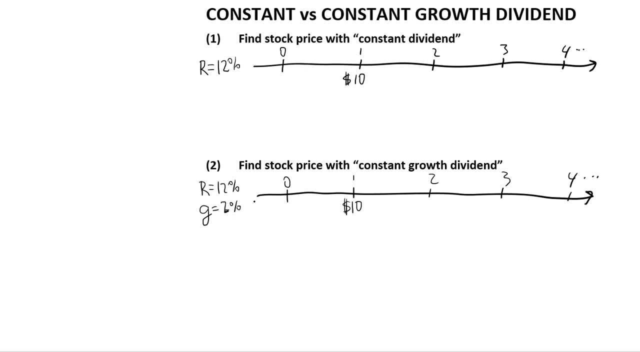 be growing every year in the future. What we want to find- let's change the color to red- is two things. So, what's the price today? And second, what's the price in two years? And we want to do the same calculations here. What is the price today? 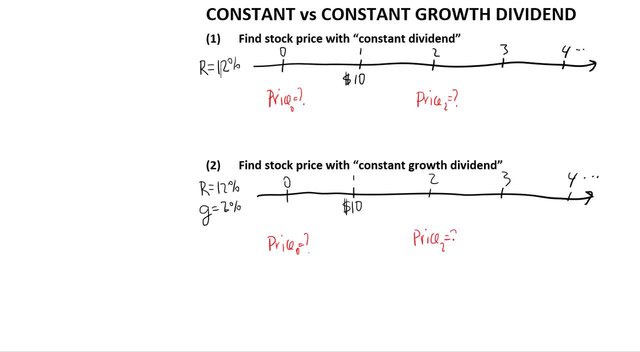 and what will be the price in two years. Okay, Let me switch to blue, which is my favorite color for all my calculations. Constant dividend, case one. Constant dividend means the dividend amount will not change, So it will stay at $10 every year forever. 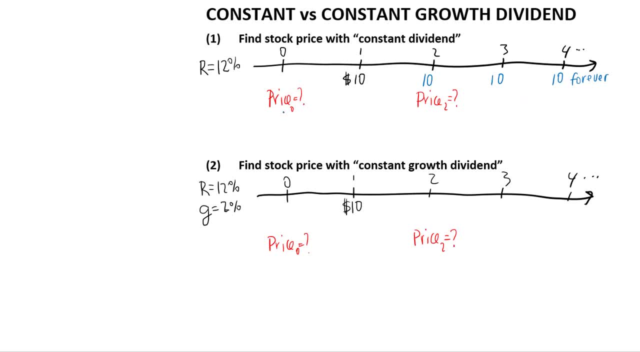 It's a perpetuity. If it's a perpetuity to find the price, so price zero, we need to take year one dividend, so D1, and divide it by the interest rate. Right. So we take this dividend, put it in the numerator. Now plug in the numbers 10 divided by 0.12.. 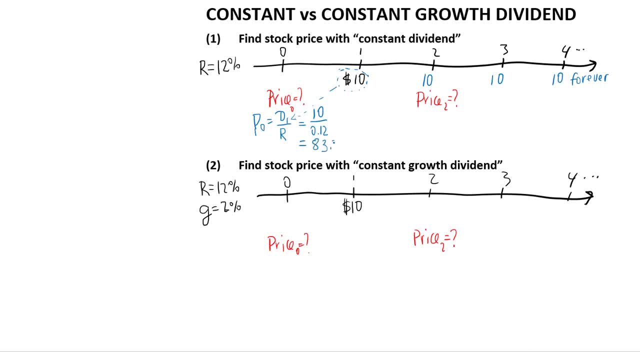 And we get $83.33 for the price that you will be paying today. that correctly represents all the future $10 dividends that you will be receiving in perpetuity. Price in two years: Same exact approach Price in year two should be calculated using the present value for perpetuity. 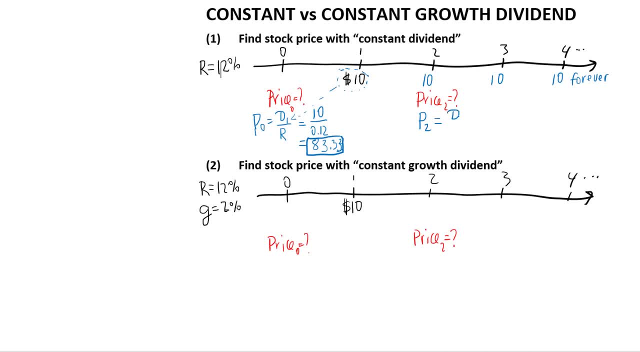 formula that says the dividend one year from this time, which is for year three, and divide by the interest rate. But in our case it's the same dividend amount. It's still $10. Every year it's $10. So the calculations will be identical: 10 divided by 12%, which gives $83.33 for the. 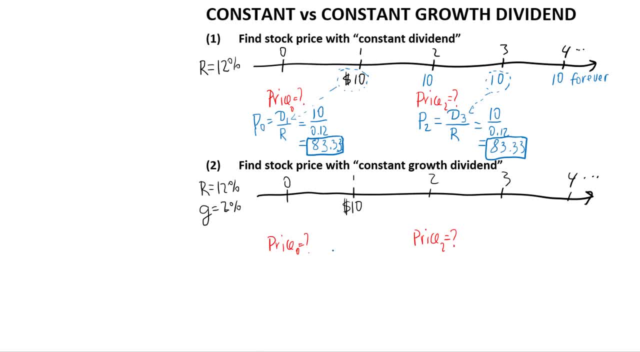 price in year two. Now we want to do the same thing in the second case, except now we added another number right: The growth rate and dividends. Why? Because this is what constant growth dividend looks like. It means the dividend will not be the same. it will. 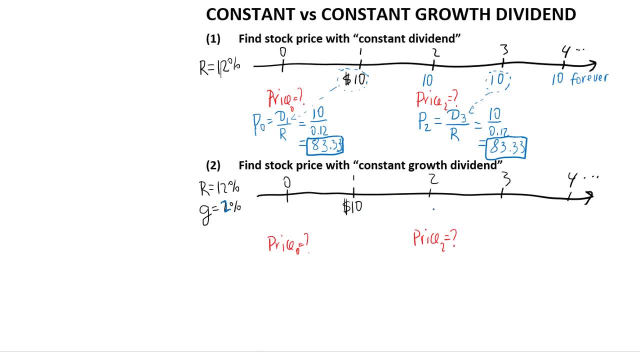 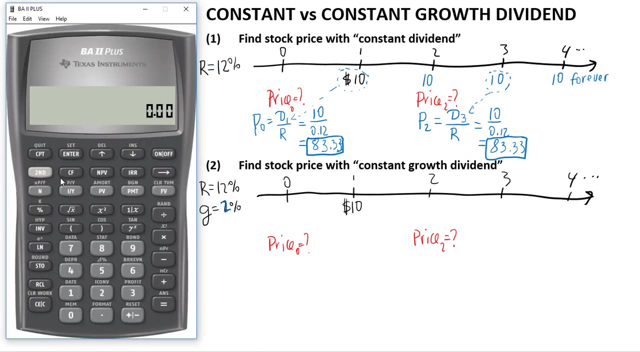 be growing at a constant rate every year, every year, forever. What will the dividend dividend be two years from today? Well, it's ten dollars in year one. We can actually use the financial calculator. Let's turn it on. Let's increase the. 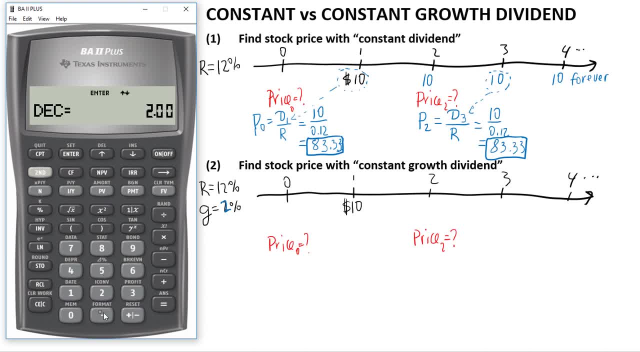 decimals. Second format, let's make it four. Let's begin Ten dollars. negative is our present value. That's in year one. We want to find what it will be one year after that if it grows by 2%. So 2% is our interest rate equivalent at. 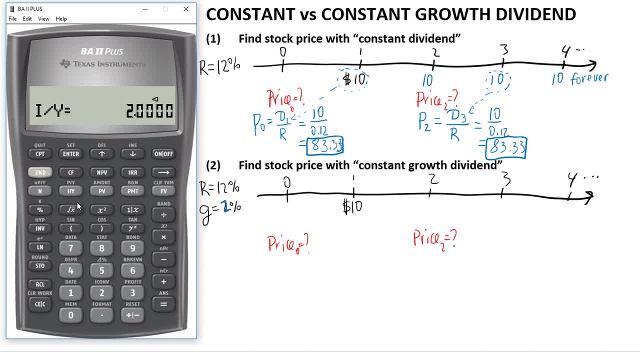 which the money grows. I press 2, IY. I want to find the future value after one year. I press 1, N and I want to compute the future value Ten dollars and twenty cents. Let's put it here, So when we 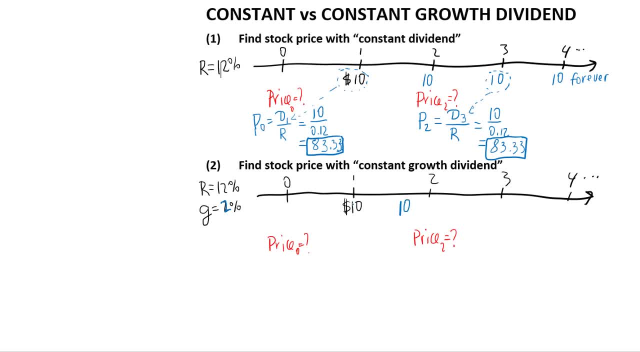 negotiate the future value. it's 10 dollars in 10 cents. Does that match our present value between 10 and 21 cents? Yes, That's exactly what we do. We basically along the different sides, we do the same thing. What we did was essentially: 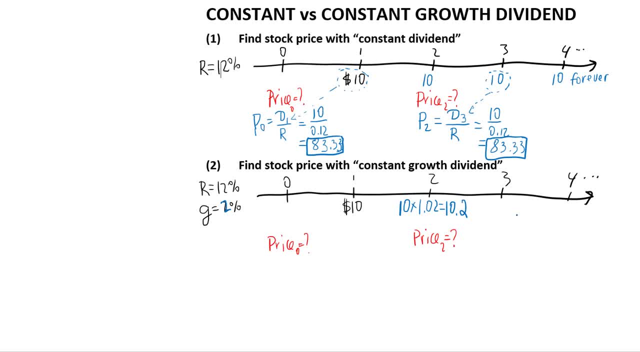 taking ten dollars from year one, multiplying by one, plus the 2% growth rate in dividends, And that's how we got our 10 dollars and twenty cents Ten point two, So that's how we got our $10.20.. Now the same way we can calculate future dividends, except we are gonna only do maybe one more, since it's going to be another perpetualiisson question, dizer. 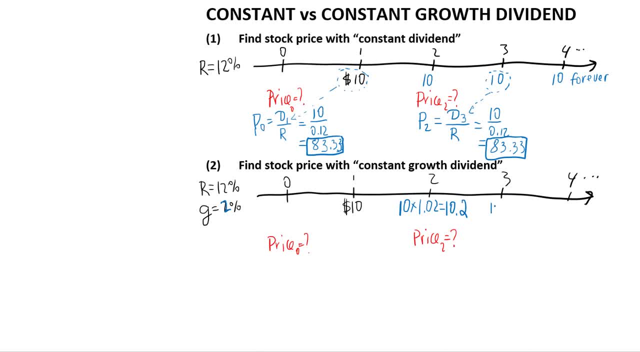 For the third year dividend. essentially you would need to do the same thing: $10.20 from year two multiplied by one, plus the 2% growth rate in dividends, so 1.02, which gives 10.404, and we can double check that. 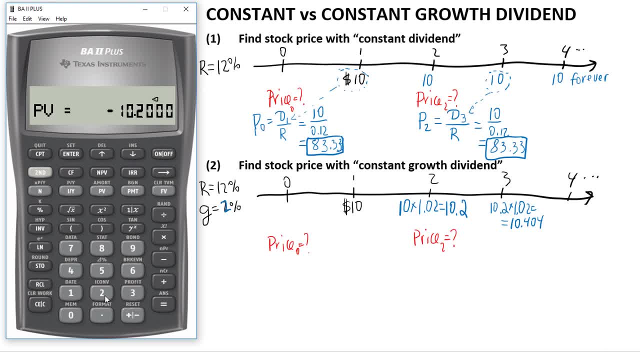 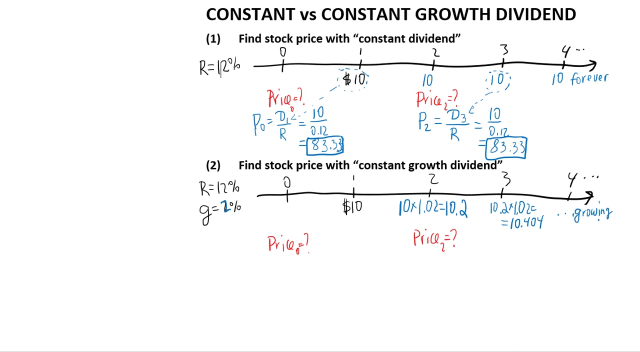 So this becomes our present value: 2% growth rate after one year gives us, compute FV, $10.404, right, So we have that number And let me put dot dot dot and call it a growing perpetuity, growing perpetuity. 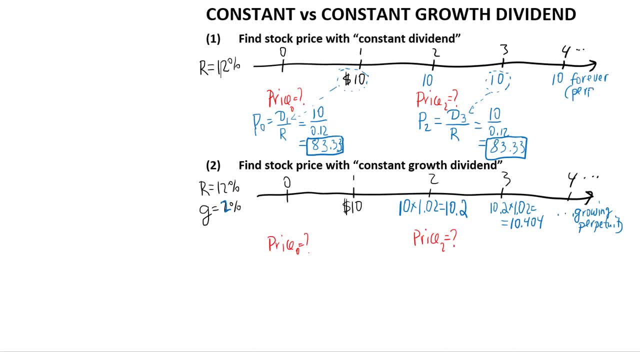 And this one here, This one here was a regular perpetuity. Perpetuity means $10 forever, every year, forever. It keeps going. okay, Now let's find the two prices. Exactly the same approach. To find the price in year zero, we need to take the dividend in year one and divide by. 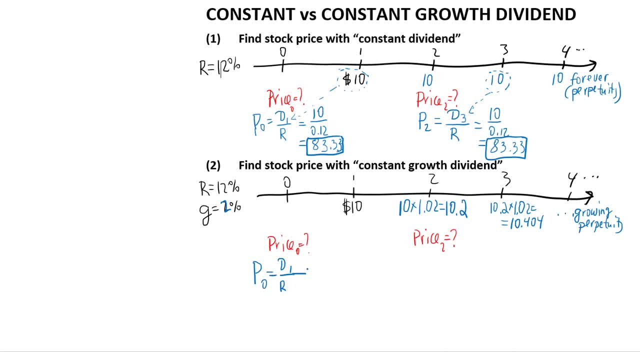 R, but this time we need to use the growing perpetuity present value formula, which is a little bit different. On the bottom in the denominator we put R minus the growth rate in dividends, R minus G, so 12% minus 2%. okay, 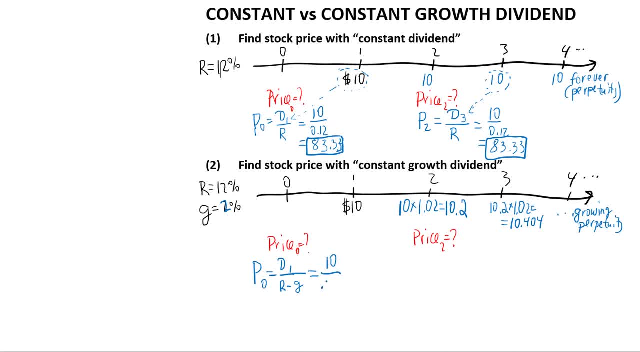 So we do 10 divided by .12 minus .02, which is $10 divided by .1, and that gives $100.. That's the price. Okay, So the price in two years is found exactly the same way. again, We take the dividend from year three and divide by R minus G. See how, for price zero we need. 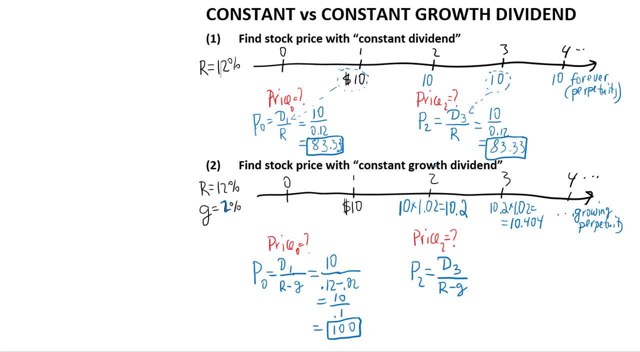 dividend one For price two. we can dividend three. We did the same thing above, except it didn't matter. All dividends were the same, They were all $10.. Here they are different amounts right Here. So the dividend in year three is $10.40 and a little bit cents 404, divided by .12 minus. 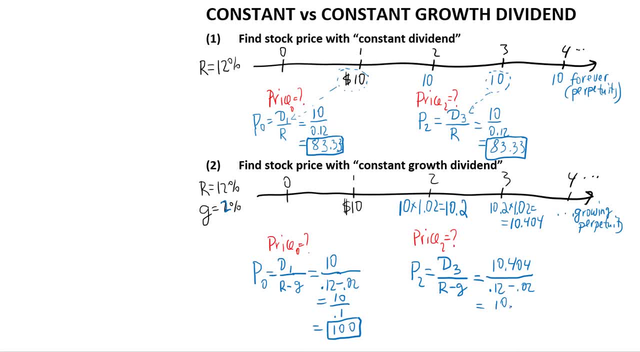 .02,, which is 10.404 divided by .1, or $104.04,. right, And you see how the price is higher two years from today compared to two years from now. right, Compared to today's price. And this is how it will always be with the stock, with dividends increasing at a constant. 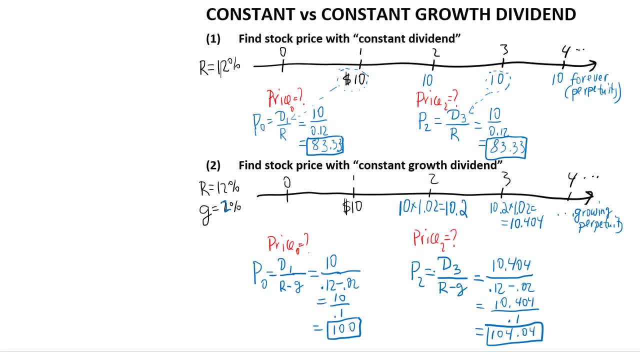 rate. And that's because, at any point of time, the price per share of stock is nothing but the present value of all future dividends after that time. And if all future dividends are larger dollar amounts, that will result in a higher price at that time. 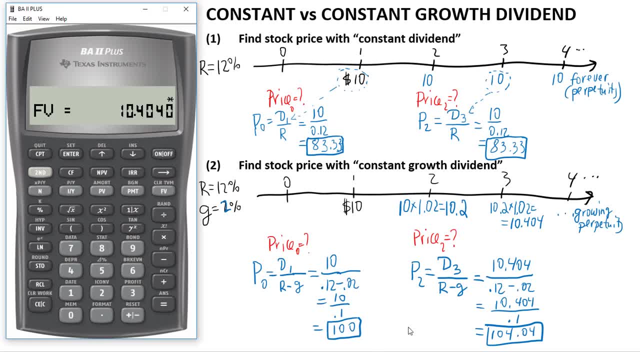 Now one thing we can notice is that this is the price today: $100,. $104.04 is the price in two years. Let's do something, Let's clear everything start out fresh. increase the decimals, let's say to four. 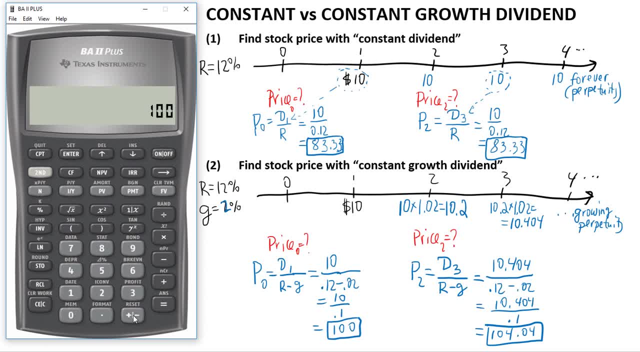 $100 negative is our present value. that's the price today. Let's say that the price in two years is two years in the future. so that's our future value. That's $104.04.. Okay, Okay, $104.04, that's our future value.